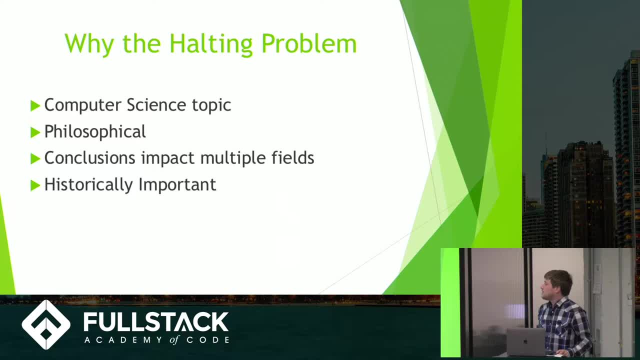 Um, it's also a very philosophical and logical kind of question and I just I love that stuff and I thought it would be really fun. Um, the conclusions of this problem impacted multiple fields um mathematics, philosophy, logic and computer science, and it's also historically important because it's one of the first problems ever to be proven. 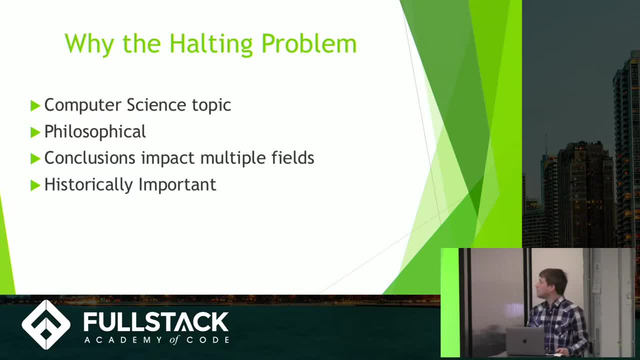 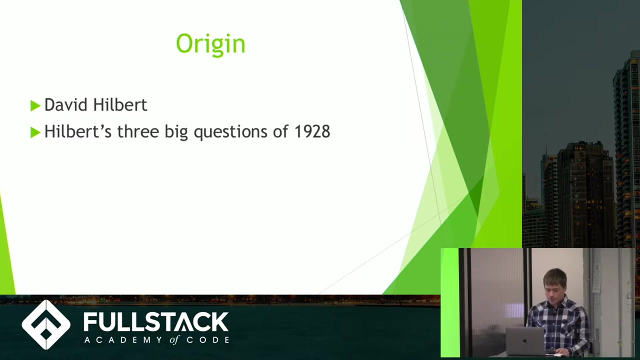 So it's um undecidable. So it's origin Um. David Hilbert was a mathematician, a German mathematician, who was very influential in mathematical logic, And in 1928, he asked three big questions, the first of which was: was mathematics complete? 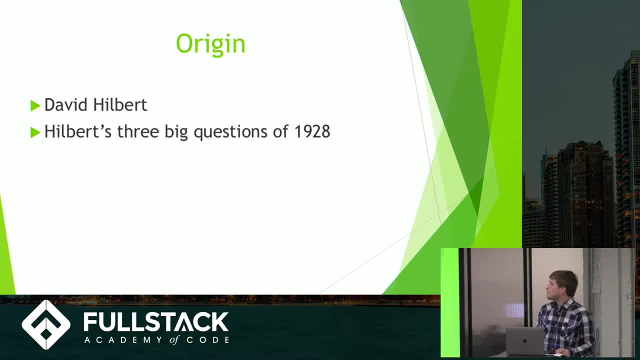 Was mathematics complete? Was it consistent? And the third, which is very important for this problem, was: was mathematics decidable, Which has a name because it's such a popular question now that it's called Hilbert's Decision Problem. Um, and once he asked this problem, a bunch of mathematicians basically started to try to make tools that could solve this problem. 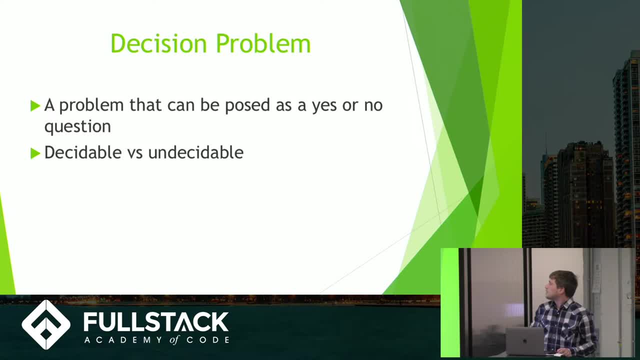 Um so what is a decision problem? Um so, what is a decision problem? Um so what is a decision problem? A decision problem is basically a problem that takes in inputs and then either responds with yes or no, And it's as simple as that. 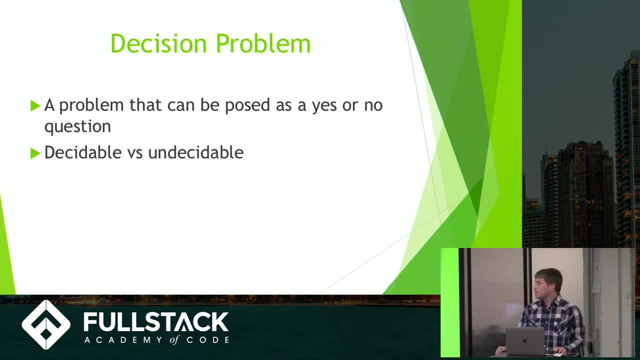 And if it can always respond yes or no, then it is considered decidable. But if in any case there is not a response that you can say yes or no, then it's considered undecidable. But if in any case there is not a response that you can say yes or no, then it is considered decidable. 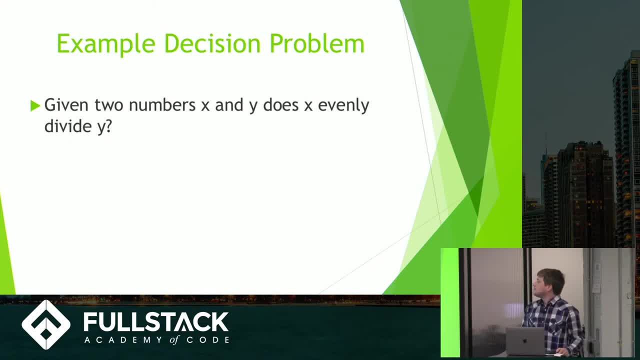 Um, so an example. decision problem is: this is a pretty simple one. It's given two numbers, x and y. Does x evenly divide y? And this is a decision problem because you're always gonna it. it expects a yes or no answer. 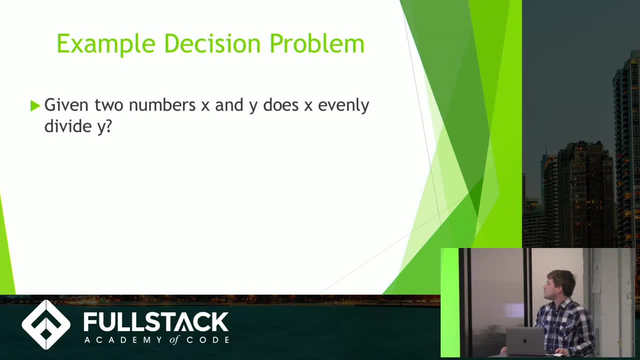 Um, so with this, you just use the long division algorithm And you take x divided by y, And you take x divided by y, And you take x divided by y, And if there's zero decimals after you can say yes, it evenly divides. 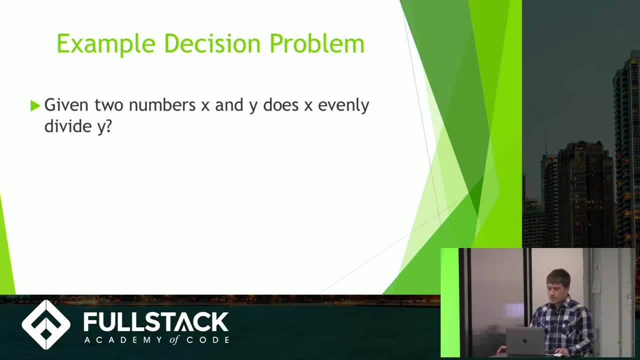 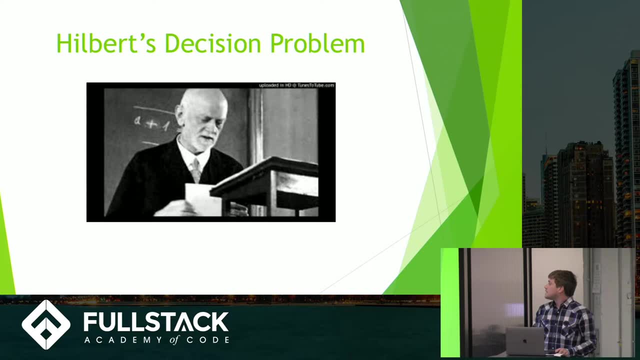 If there's decimals, you say no, And since you always get a yes or no, it's considered decidable. Hilbert's decision problem basically just like that, just a little more complicated. He asks um if there is any algorithm that can basically look at any first order logic. 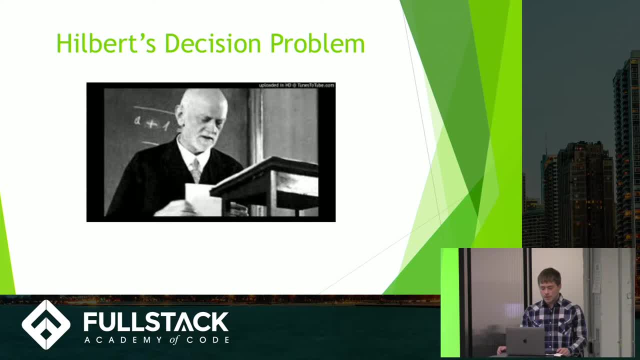 And always say yes or no if it's completely valid. Um which, if he could do so, it would basically be able to um verify algebraic equations, integration in calculus or the truth of a derivation in logic, And this inspired a lot of people to really tackle this. 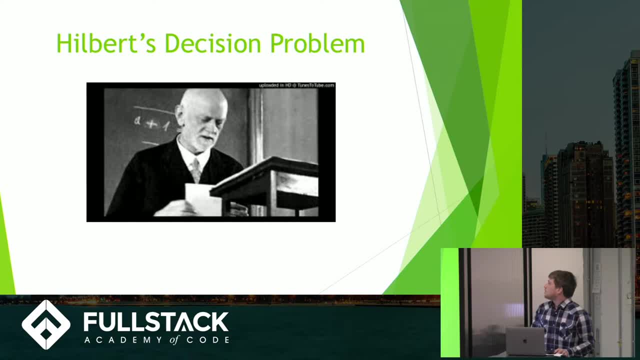 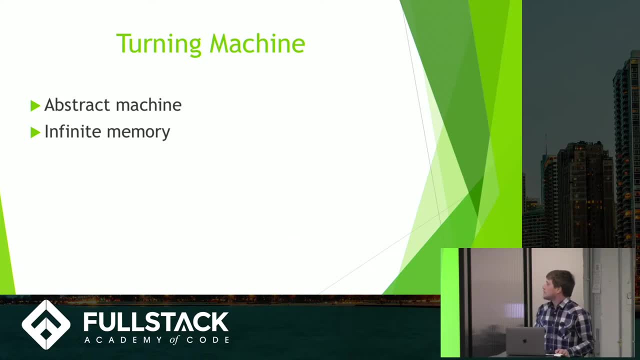 And this inspired a lot of people to really tackle this. And this inspired a lot of people to really tackle this, Uh, which also helped lead to the turning machine, which is an abstract machine which, uh, basically reads off a tape and follows a specific set of rules. 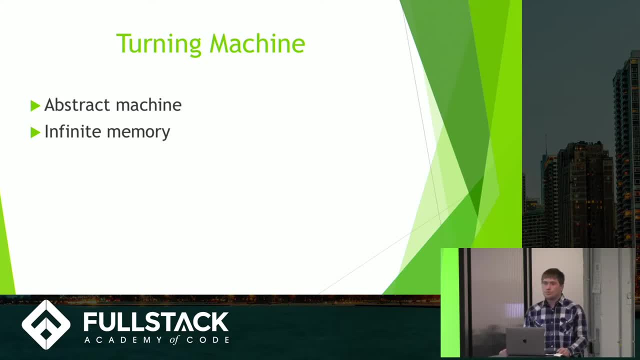 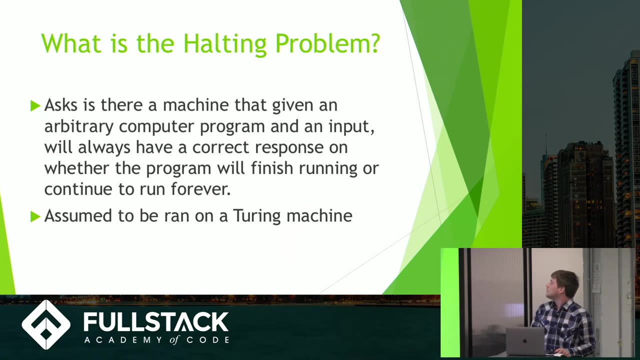 And it can be constructed to uh basically simulate any algorithm. And what's very important- for once we get into this problem- is it has infinite memory. So what is the halting problem? It's basically just like uh Hilbert's decision problem, except it asks: is there a machine that, given an arbitrary computer program and an input, 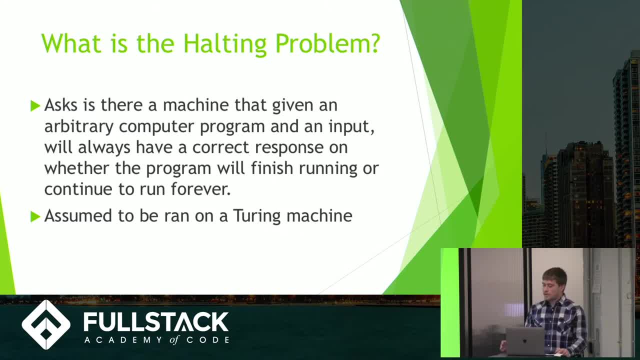 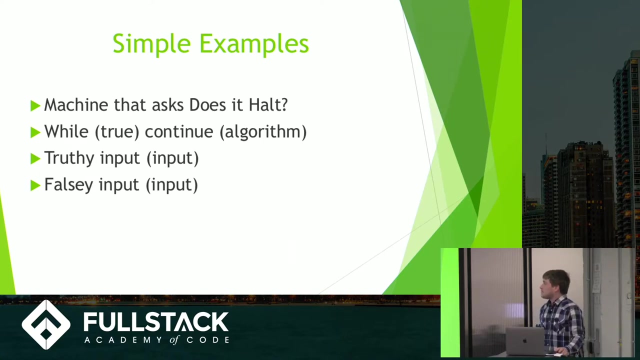 will always have a correct response on whether the program will finish or will it run forever And not finish, And it's important that this is assumed to be on a turning machine, because then it will run infinitely And we'll get into that. Uh, so a simple example of how this would work and how you can see an answer to this is: 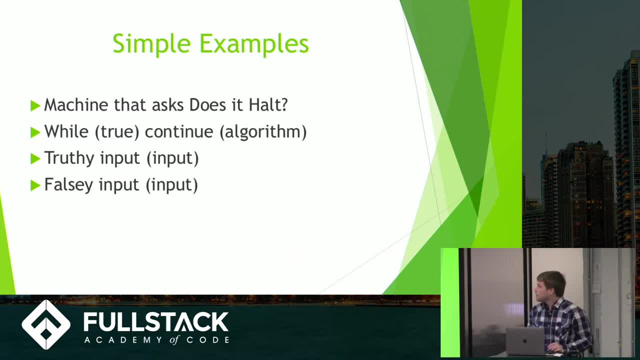 you have a machine and basically it has some crazy algorithm in it And it, uh, it asks: does it halt? And it will respond with yes or no. And so the program we're gonna input is, while true, continue, which is the algorithm. 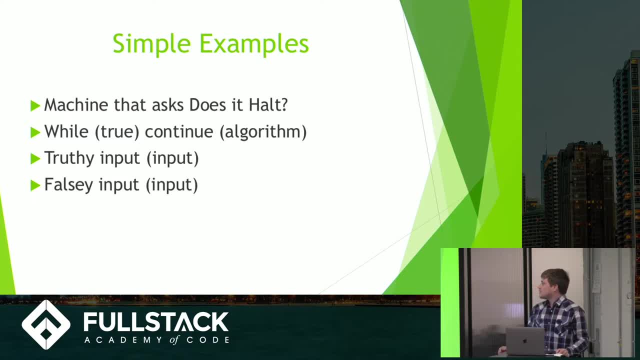 And then the first input we'll try is: if you put in something true, you'll see that it'll run forever because it'll just keep looping through and never end. So the machine would be able to say yes, uh or no. 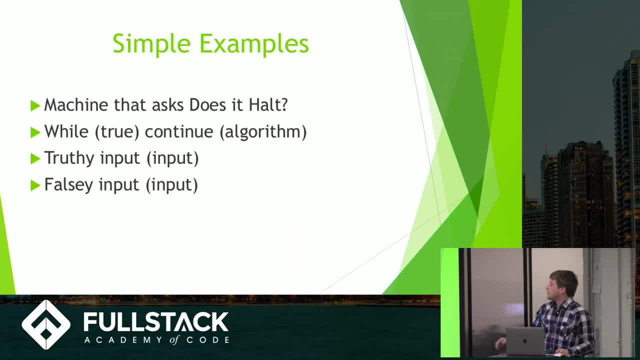 This will never halt And if you put in a false input, it it's pretty simple to see that it'll just stop and the machine will say, yes, this will halt. But this is pretty, this is pretty basic What. what would happen if we have much trickier things that aren't as easy to see as this? 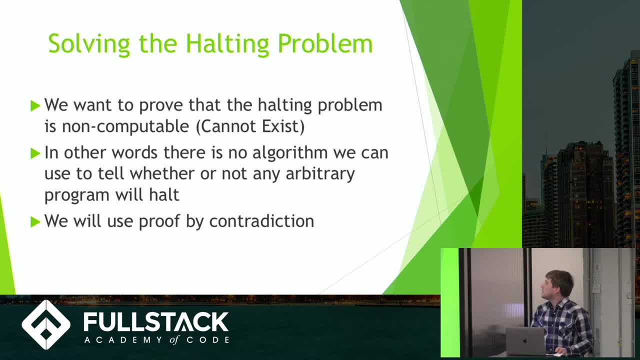 Um, so, in order to answer that, we have to get into solving the halting problem, And to do that, we want to prove that the halting problem is non-computable, And if that's the case, it cannot exist. 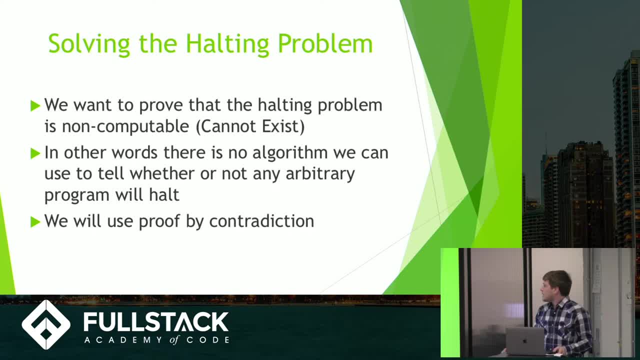 So, in other words, we want to show that there's no algorithm that we can use to tell whether or not any arbitrary program will halt, And to do this we'll use a proof by contradiction, which is what Alan Turing did in 1936.. 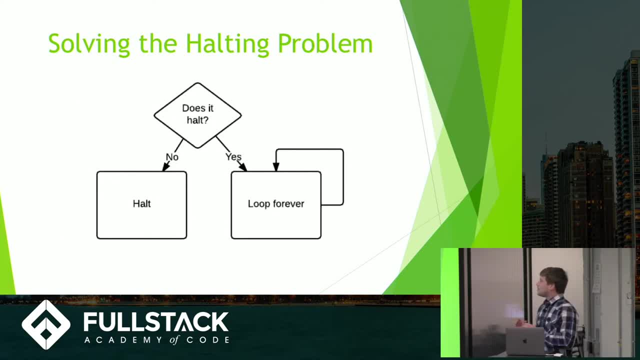 So basically we take that original machine with that crazy algorithm and we're basically just putting it as a decision box for simplicity. And, if you, what it does is it takes in the program and input and it says yes, it halts, or no, it doesn't. 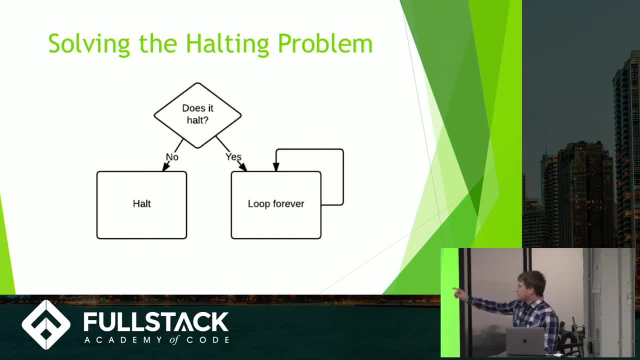 And by simply adding at the end of it: if it- if it says yes, it does halt, we're going to add a loop that goes on forever. And if, no, it doesn't halt, we're going to add that it halts. 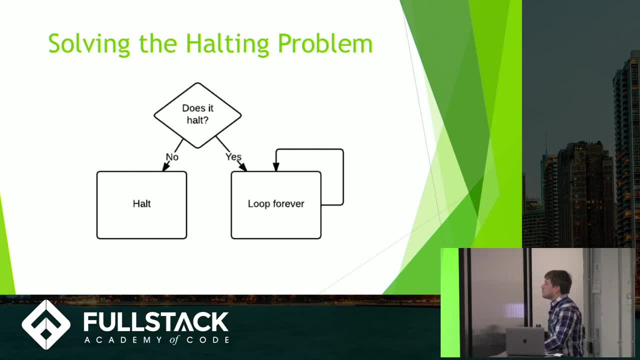 And this is pretty cool because if you then take this machine and feed it to itself. so you ask: does this machine halt when fed to this machine? And what happens is that if the machine, which is supposed to always give you a right answer, 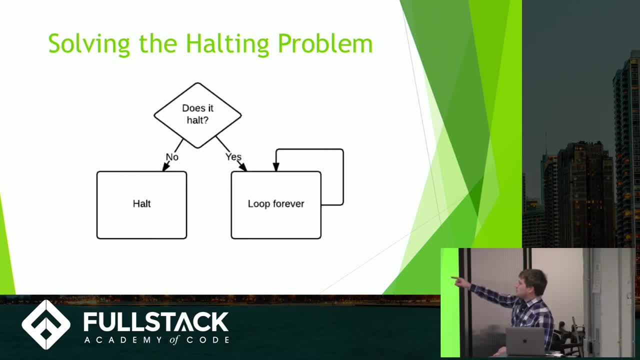 says yes, I do halt, it then loops forever and contradicts itself. But if you say no, I don't halt, then it halts and also contradicts itself And through this contradiction basically show that this machine cannot exist and there exists no machine that can accomplish what 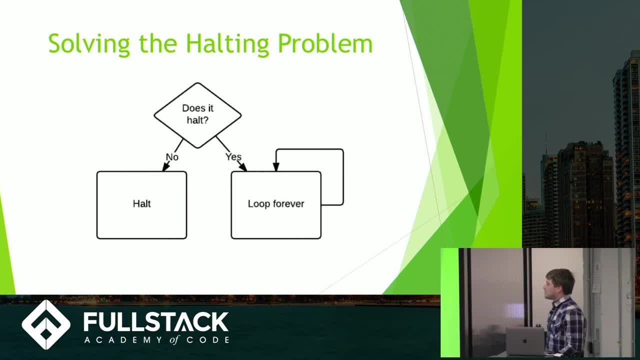 uh, the halting problem machine was trying to accomplish And it this can be kind of confusing, and a more simpler way to think about it is, um this: what happened at MIT in 1986, a professor asked his class: 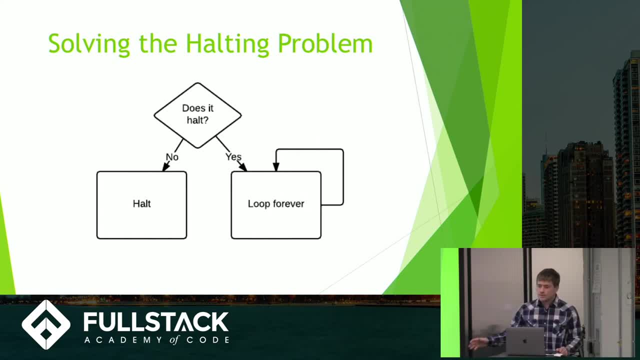 uh, at the, as he's getting ready to end the class, he says: is there any last questions? And a student asks: will this be the last question? And basically it's a very clever question because no matter what the professor says, 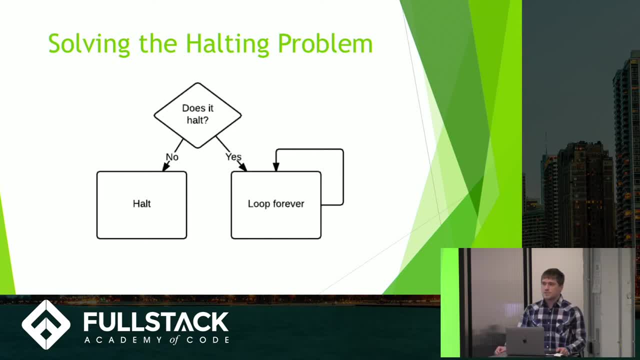 the student then has the opportunity to contradict him. So there, there can never be a valid answer to that question, Because if the professor says yes, this is the last question, the student only need ask one more question. But if he says no, this is not the last question. 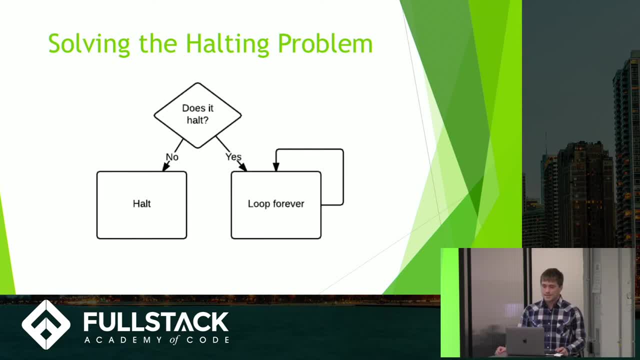 the student just need not answer another question or ask another question And basically it just proves that computers and humans can't do everything or solve everything. There's perfectly valid questions that it will never be able to answer. Um, so what are implications of this? 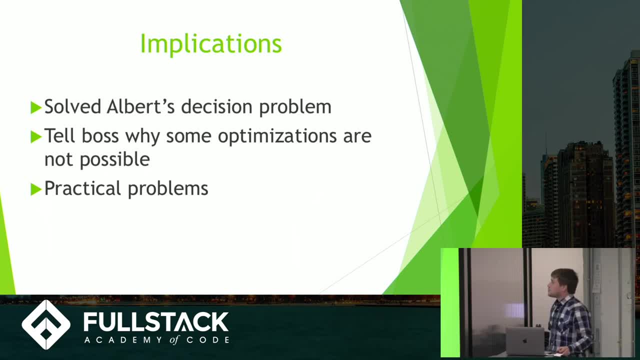 It solved Albert's decision problem, which was very impressive in itself, And it also like, if you're in the workplace and your boss asks you to basically make some very general optimization that can cover everything, you can tell him you can't do that. it's impossible.